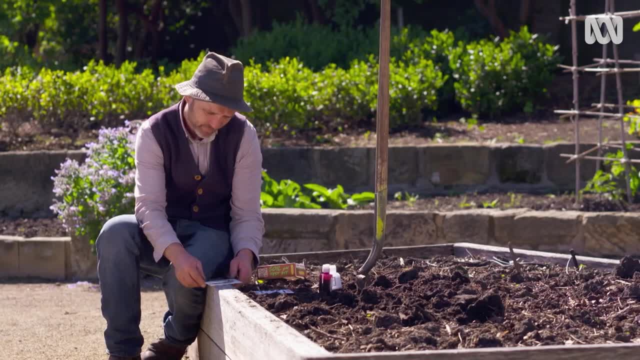 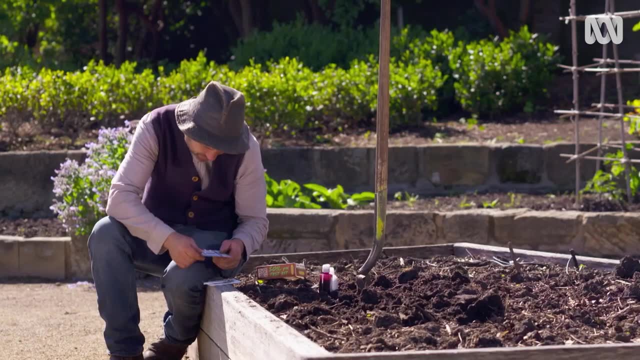 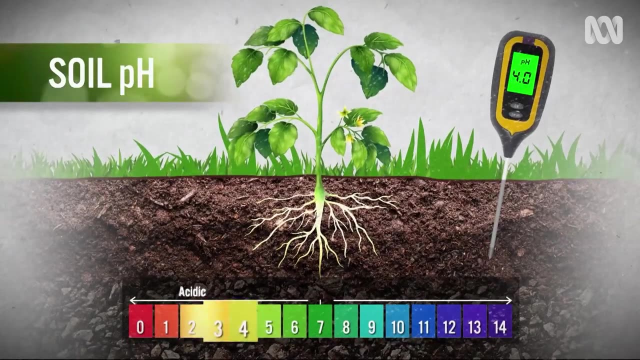 Then add some barium powder and wait for the colour to change. The pH here is 7, which is neutral, which is a perfect place to be in your garden, and here's why, As the scale of pH changes, so does the combination of nutrients available At the centre of the scale, the most important. 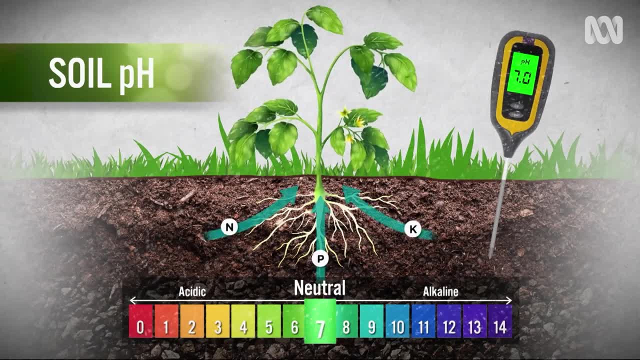 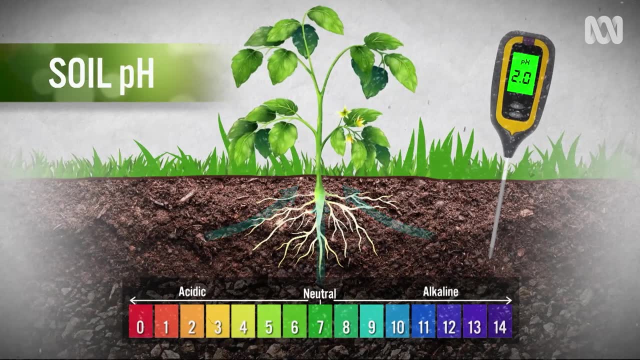 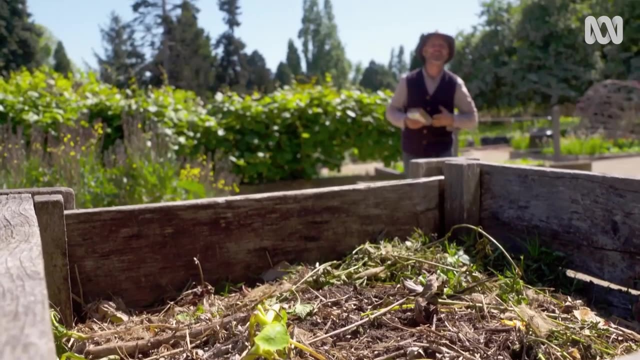 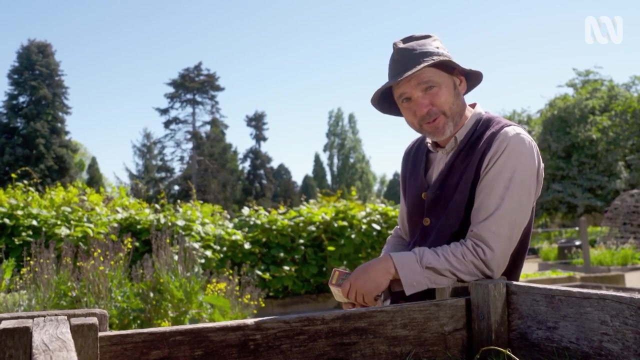 nutrients like nitrogen, potassium and phosphorus are most readily available for plants to take up. At the pH extremes these become less available and other elements like aluminium can become toxic to your plants. It's a really good idea to take multiple soil samples from different parts of your garden and do it before you add compost or any minerals and make 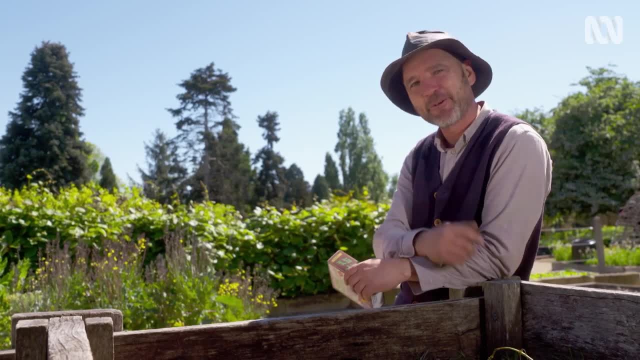 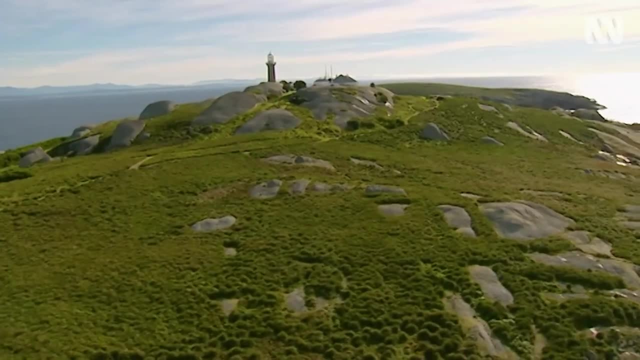 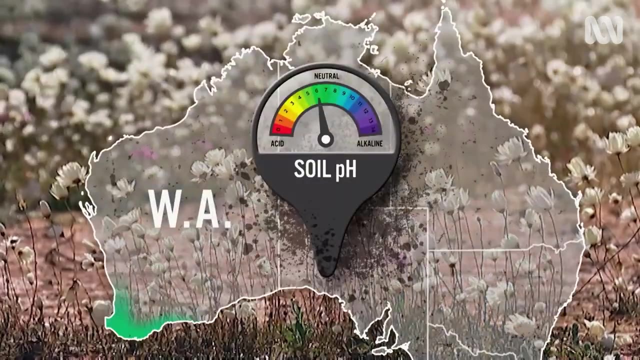 sure it's on a nice dry day. That way you'll get an accurate reading. There are general patterns of soil pH around Australia based on things like the type of underlying bedrock, agricultural use and the amounts of rainfall. Much of Western Australia's coastal regions are alkaline due to the presence of 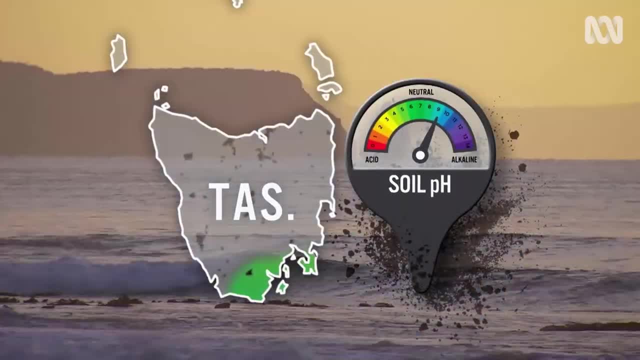 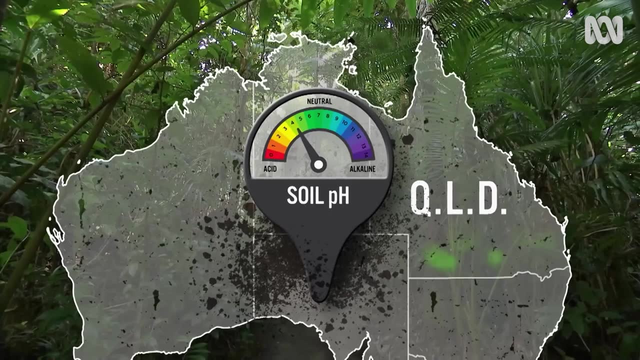 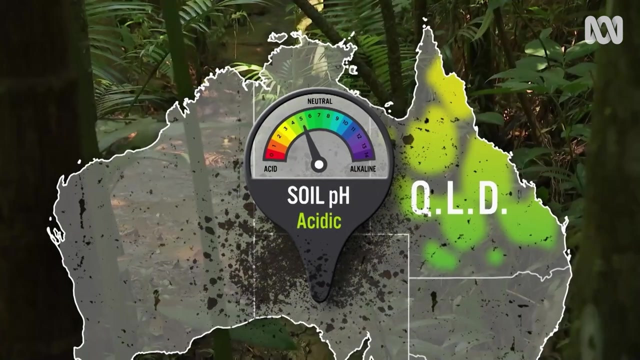 limestone. On the other hand, Tassie's east coast is dominated by dolerite clays getting more acidic as you head north. Whereas two-thirds of Queensland's surface soils are considered acidic, This is due to rainfall and the constant leaching of certain nutrients. Dryer areas are more alkaline, as the 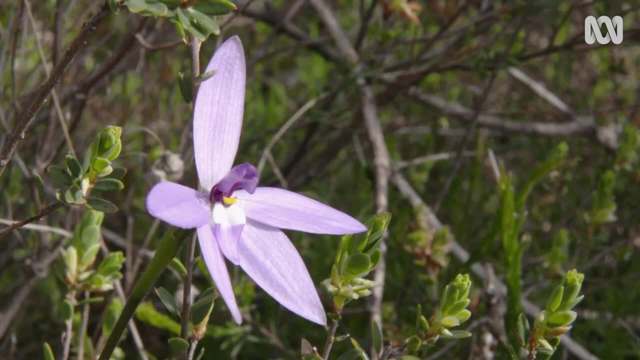 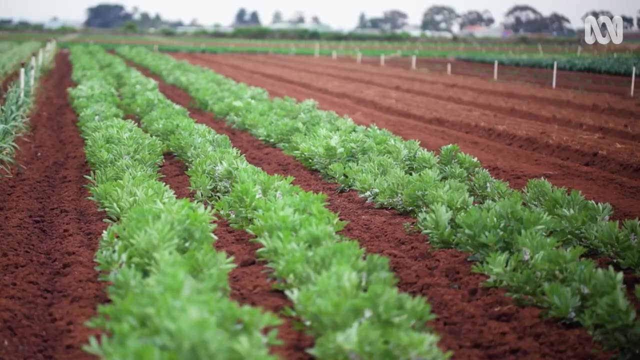 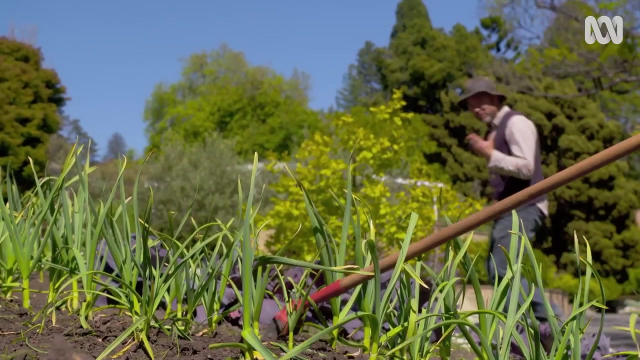 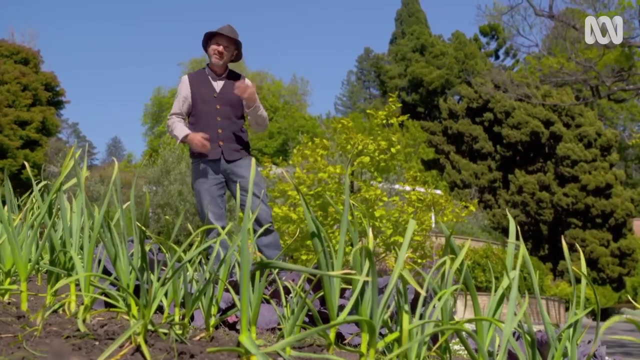 combination of elements in the soil are more stable And 50% of Australia's agricultural lands have high acidity due to practices like using ammonia heavy fertilisers. At the higher end of the pH scale are our alkaline soils. A pH of around three to eight is perfect for plants like brassicas, garlic, spinach, hibiscus, sweet peas. 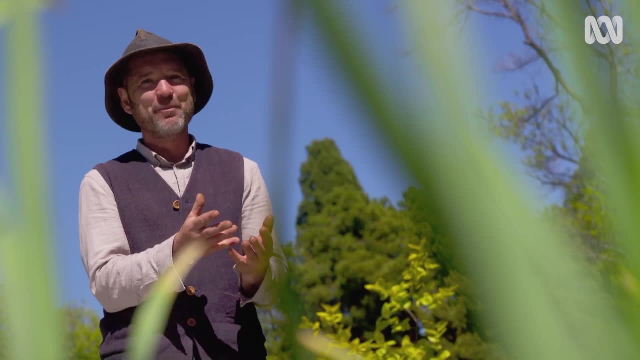 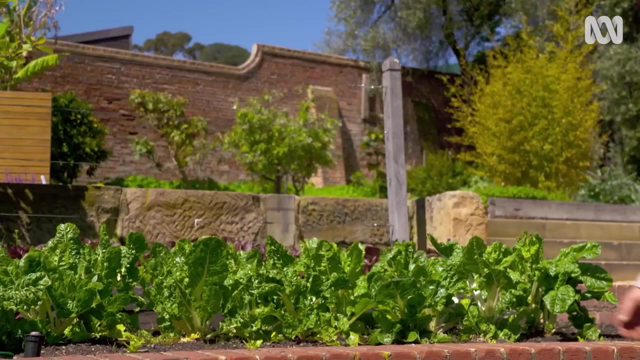 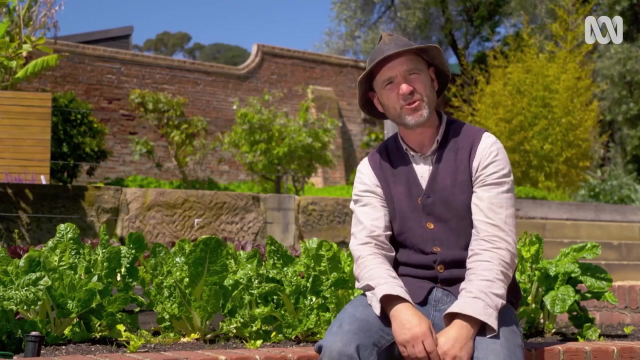 and geraniums. At this range, all the major elements, plus more calcium and magnesium, are available, which is a diet that these plants prefer. Most of your veggies like to sit about mid-range six to seven, which is close to neutral, and that makes a lot of sense because they're